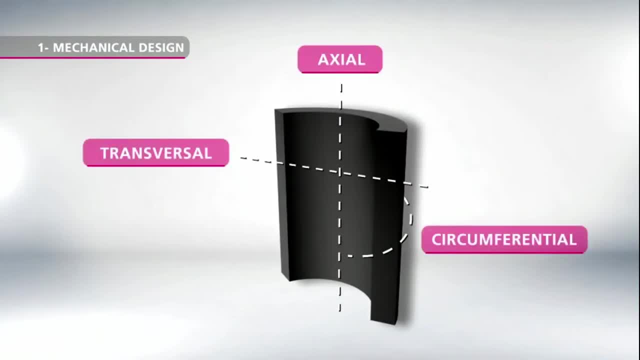 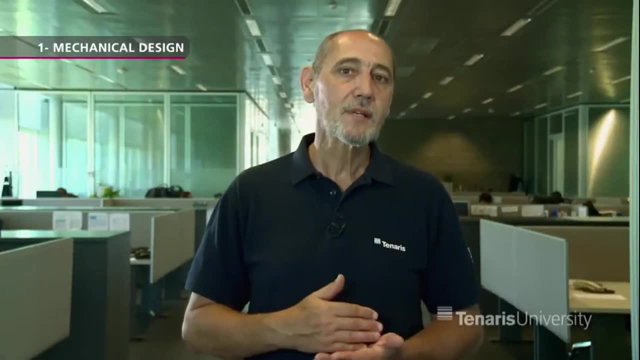 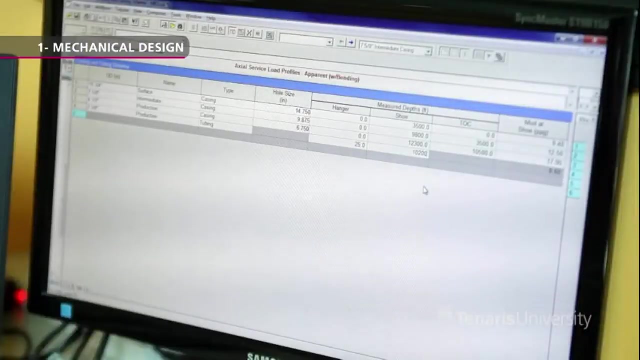 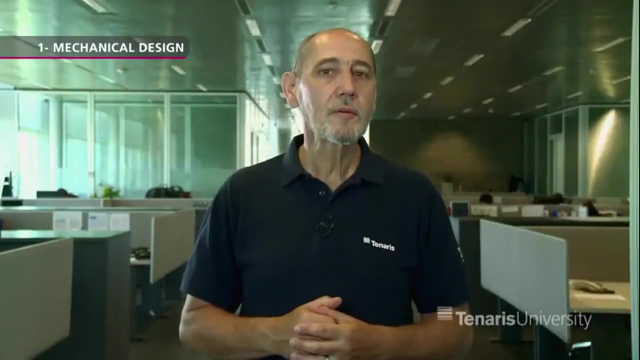 transversal and circumferential, known as von Mises. This design involves the use of complex formulas that can be easily solved through different software available in the industry. Input information is required to fit this software. This data includes some general information about the customer and the location, and specific information related to the. 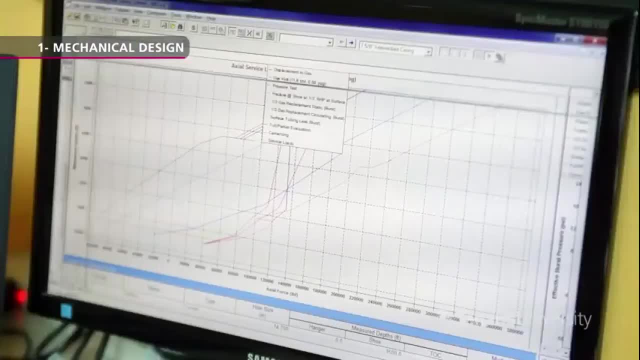 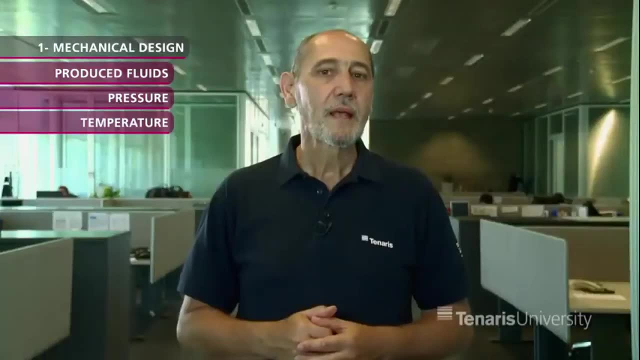 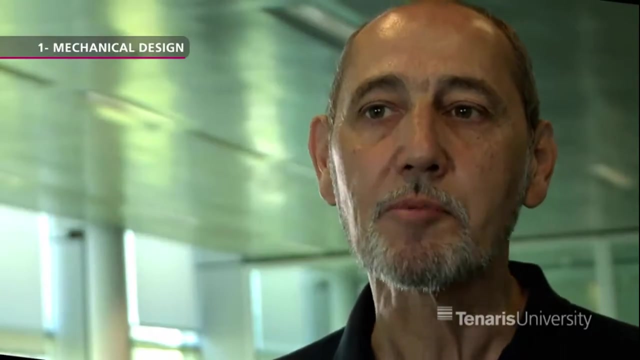 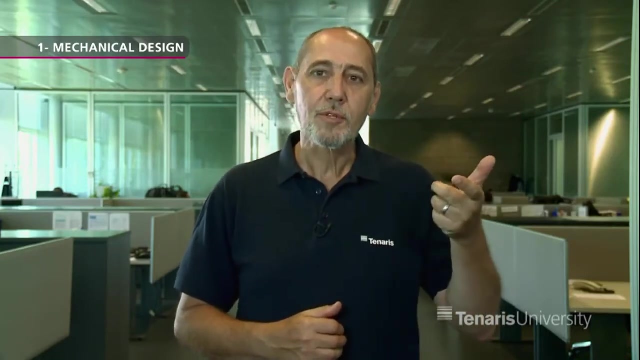 characteristics and the type of the well, including composition of the produced fluids, pressure, temperature, as well as other parameters if they are available. Additionally, the purpose and depth of each string to be designed must be specified. Remember, when we saw OCTG products, we had said the string design would be specific for each. 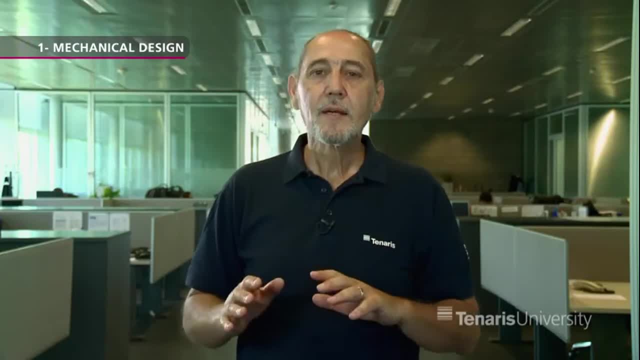 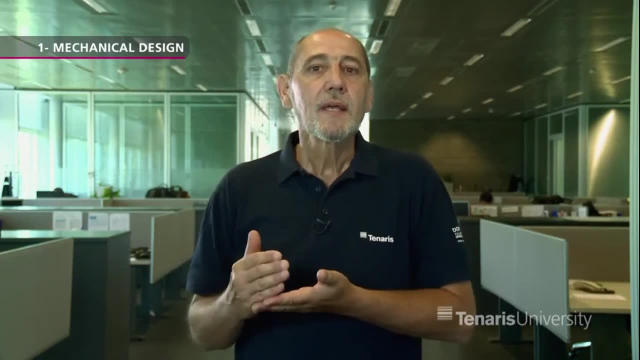 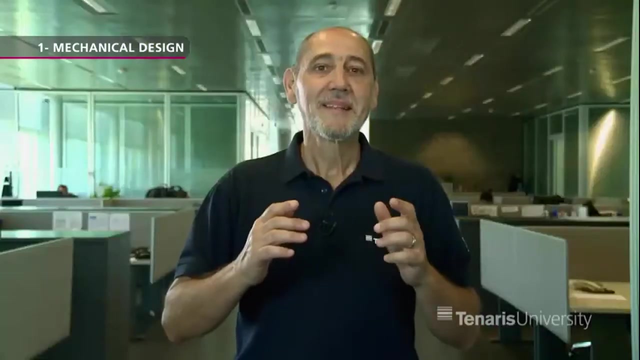 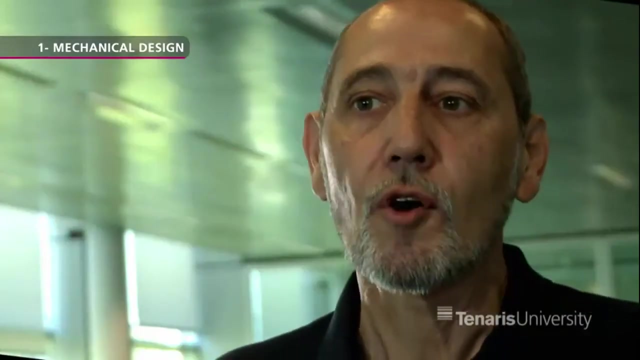 particular use of the pipe. It is completely different to design, for instance, a 5 1⁄2 string if it would be using, as a production casing, a drilling liner or tubing. The loads to which such strings will be subjected will on their use and, as a consequence, that their design factor will be different. okay, once the 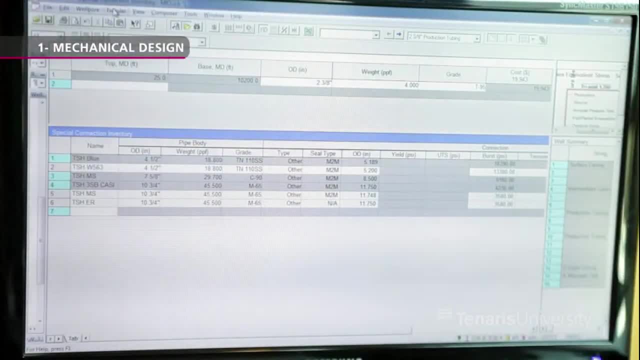 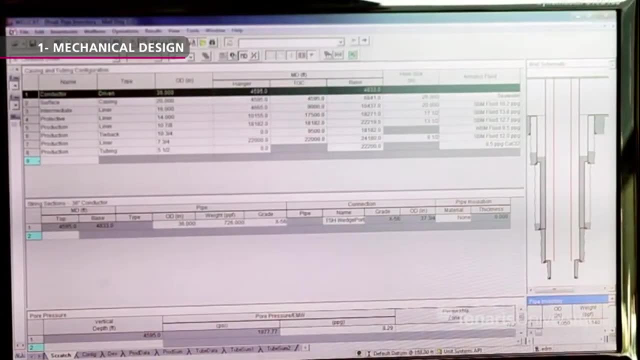 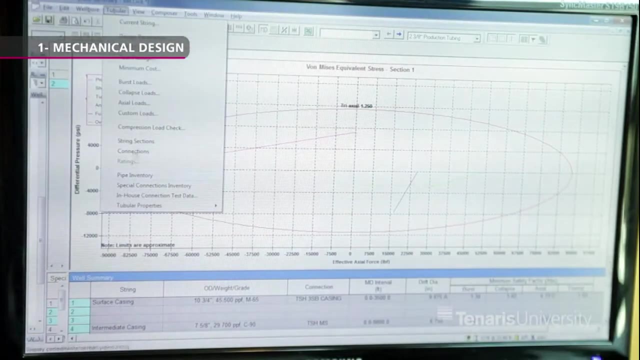 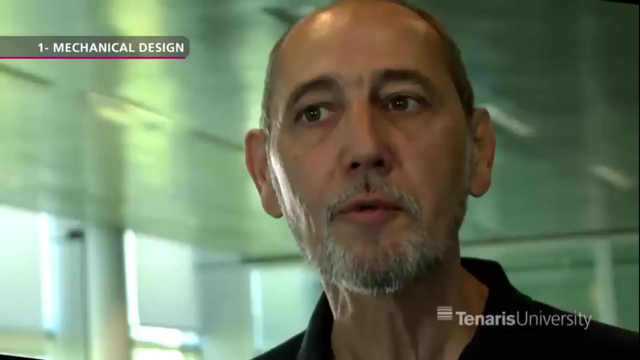 information is entered into the system, the designer must define different load cases, which represent events that the designed strings would eventually face during their lives inside the well. for this operation, the well conditions must be analyzed in deep detail to determine the proper load cases that better describe such situations. the output of this process is a graph. 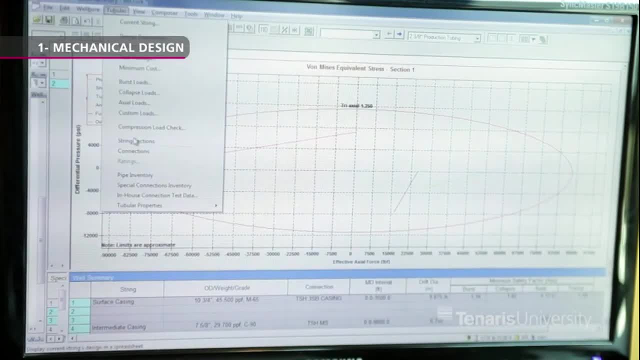 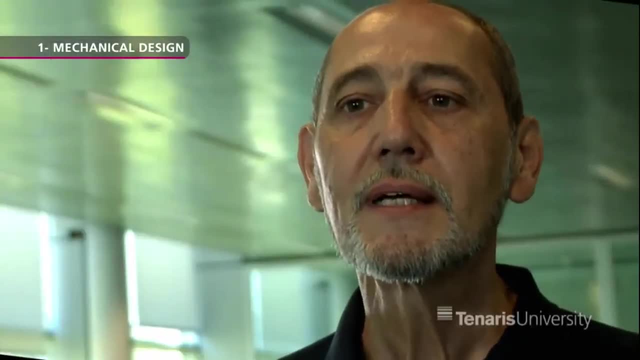 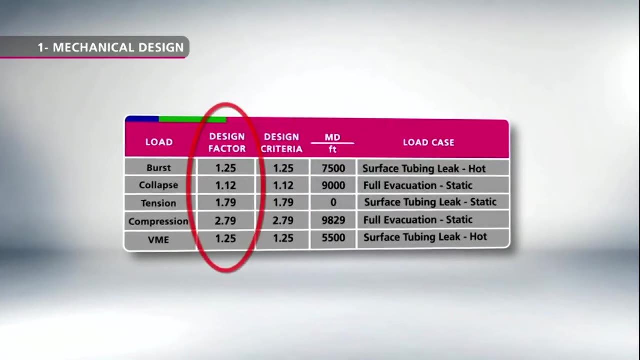 with the service envelope of the selected pipes and the stress is produced by the different loads. considering the design, additional to the graph, the design factors calculated for each of the five different loads, which is the pressure получить the load and the effect factor, design parameters, burst collapse, tension, compression and bond misses are.